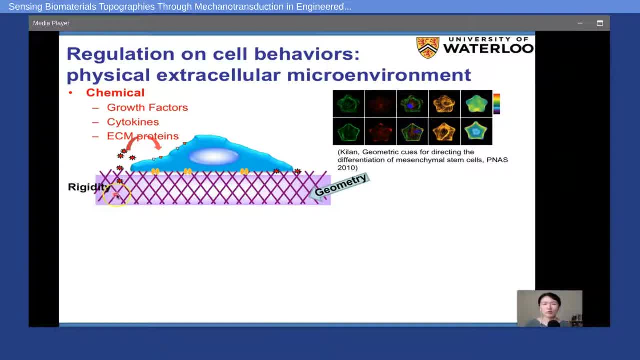 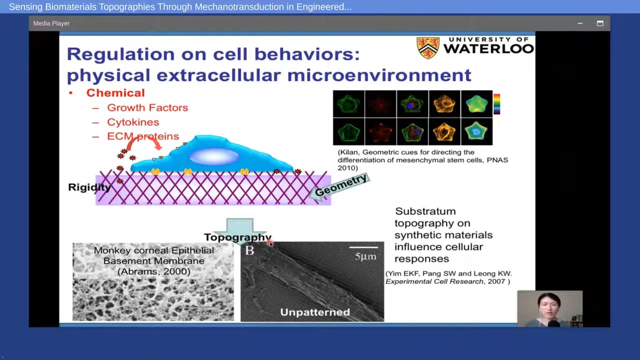 also show us that mechanical factors, such as the rigidity of material or by controlling the geometry of cells, could also affect cell's behavior. Our lab is particularly interested in the topography of the extracellular matrix, And we, as well as other groups, 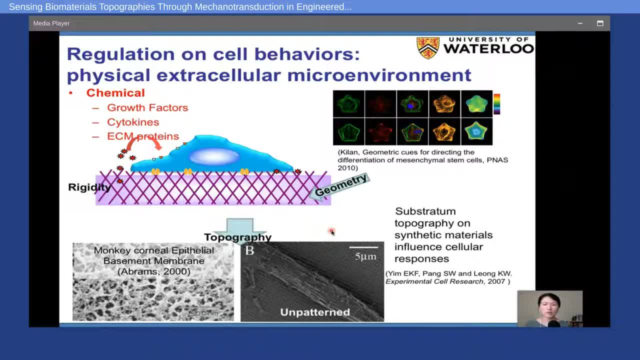 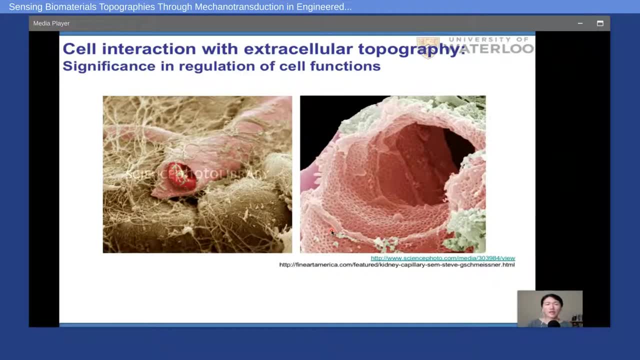 have shown that this substrate topography, when we replicate on synthetic material, this substrate topography could affect different cell response And in fact this type of extracellular topography can find in many types of tissue. These two pictures are two electron micrograph pictures. 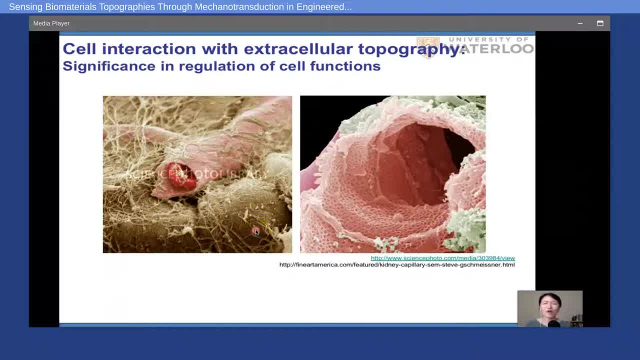 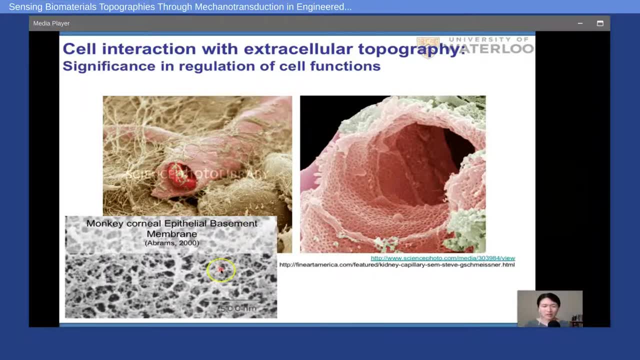 I find from the internet, But it shows a very rich reservoir of extracellular topography found in the vasculature. Another electron micrograph picture shows here is the topography in the corneal epiphyllal basement membrane. So this evidence shows 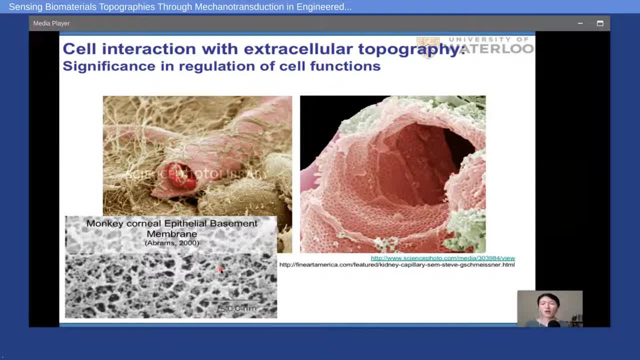 that cells are surrounded by a rich reservoir of extracellular matrix. So this evidence shows that cells are surrounded by a rich reservoir of extracellular matrix. So this evidence shows that cells are surrounded by a rich reservoir of extracellular matrix. Our lab is interested. 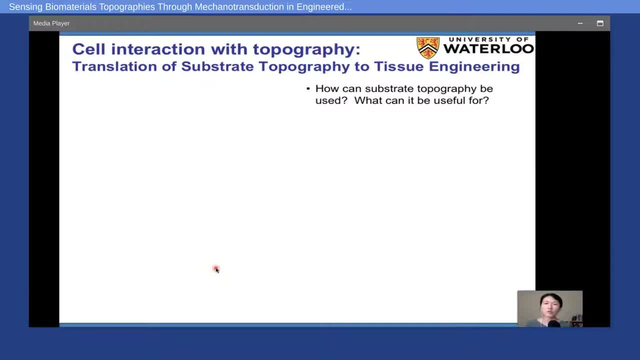 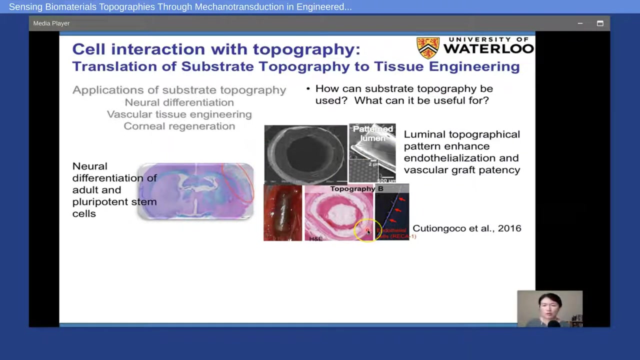 in applying this type of topography for a tissue engineering application. So how can we apply this topography? for We have been working on different type of applications, So we have been interested in applying the topography on neuronal differentiation, vascular application or vascular repair. 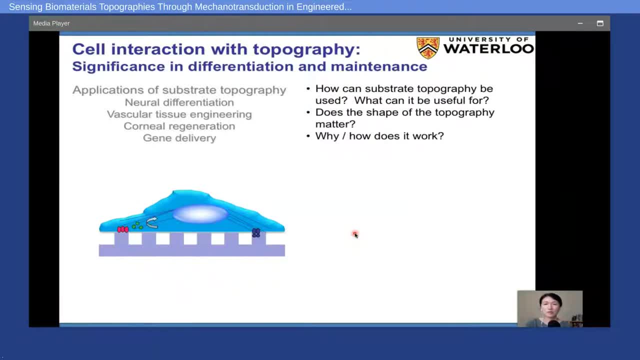 as well as contact line corneal regeneration. For today's talk, I will be focusing on talking about how does it work, or why does it work? Our group has been looking into the mechanobiology in the topography-induced cells behavior, including 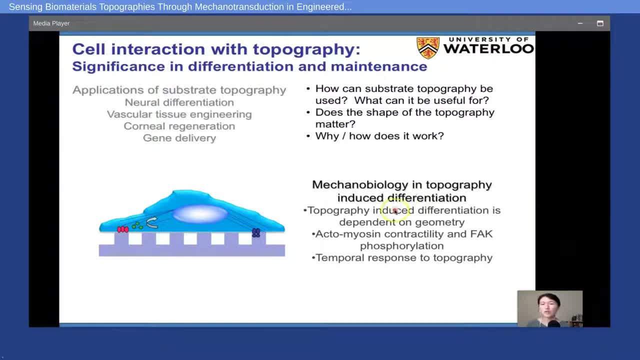 topography-induced stem cell differentiation. We find that topography-induced differentiation is dependent on the geometry of the pattern. An important component of the topography sensing is the actin-marsens contractility and the focal adhesion signal. So before I start talking, 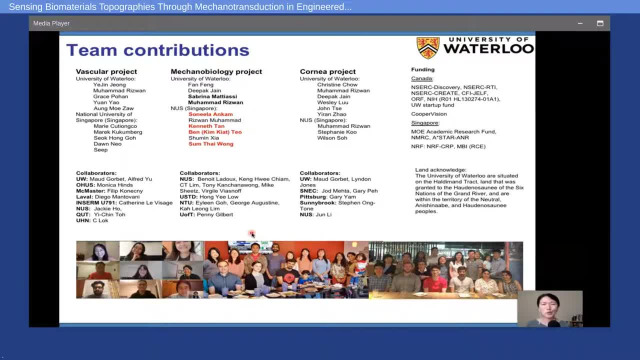 about the data today. I would like to acknowledge the contributions from my research team as well as our collaborator, So I highlight that member of my student and postdoc who has contributed directly to the presentation I'm going to give today, and also 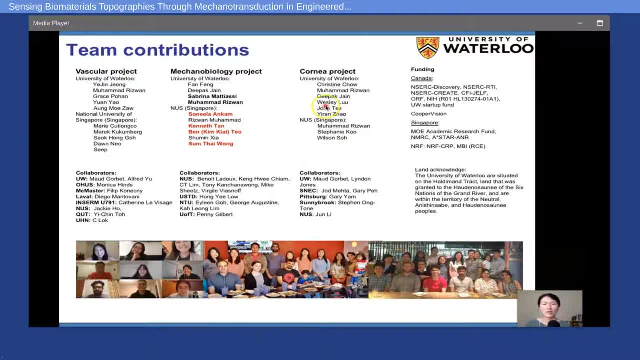 show some other of my lab members, both at the University of Waterloo and also in the National University of Singapore in Singapore. So I have been a principal investigator in the faculty in the National University of Singapore before I relocated to the University of Waterloo in 2016.. 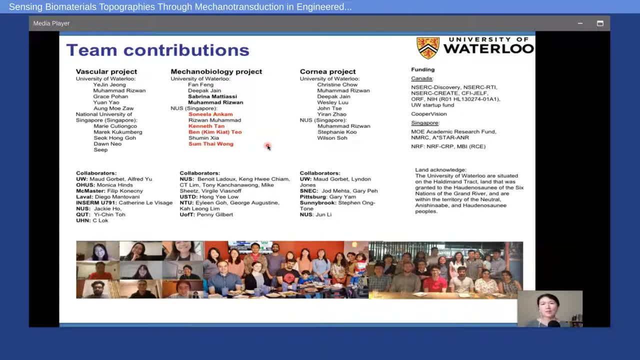 So some of the work I show today are also generated from my former lab member from Singapore as well. In addition to my lab members, I would also like to thank and a lot of my fellow collaborators, as well as the funding source that enable us to do the work. 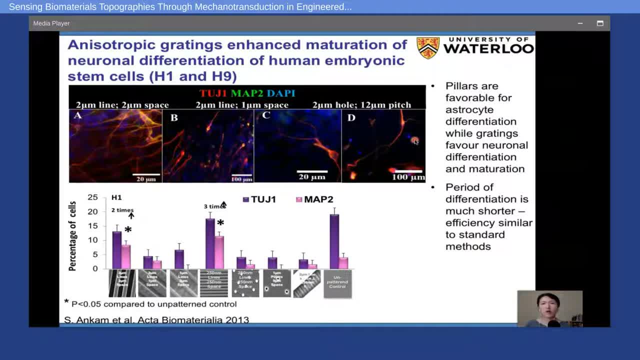 We start investigating the effect of topography on stem cells differentiation, on the effect on the neuronal differentiation. So in this study we cultured human embryonic stem cell H1 and H9 on different type of topography. In general we find that pilar substrate usually 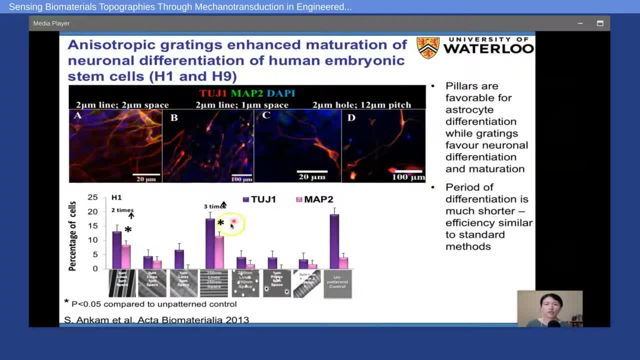 will favor and enhance astrocyte differentiation versus grating substrate, will prefer or favor to neuronal differentiation, And they will also enhance neuronal maturation. The period of time required for the neuronal differentiation is usually shorter than compared to unpatterned substrate or other protocol using. 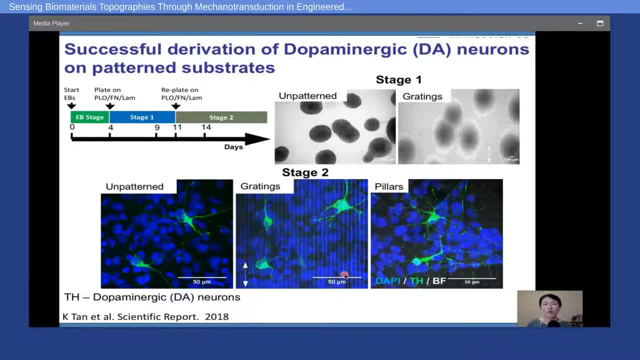 unpatterned substrate. We have also investigated how to divide neuronal subtypes using a combination of topography with other protocol. My former postdoc, Kenneth Tan, has taken this work to differentiate induced polypotent stem cells through a two-stage protocol. 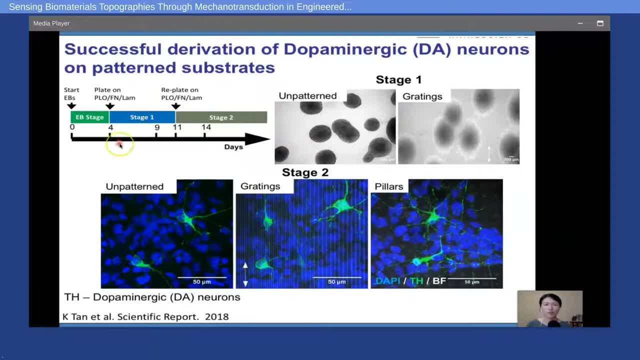 And then he incorporated topography in stage one, which is the lineage commitment stage, as well as stage two, which is the maturation stage. We find that while in stage one, in lineage commitments, that gratings do enhance the neuronal differentiation, in stage two 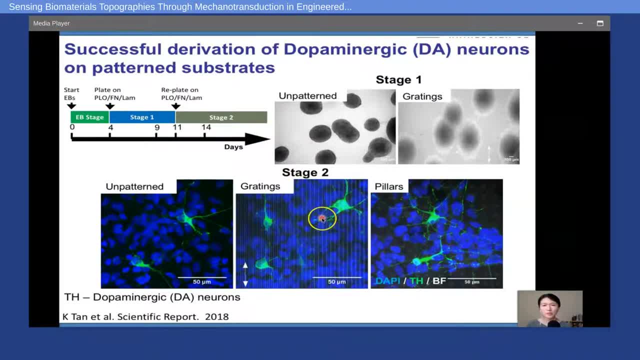 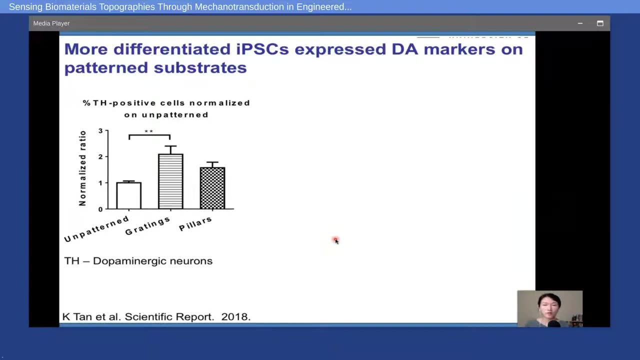 in the maturation stage. both gratings and pilars will also help to enhance the maturation and derivation of neurons, To investigate or to examine the derivation of topomunergic neurons. we take the information, we take the information, we take the. 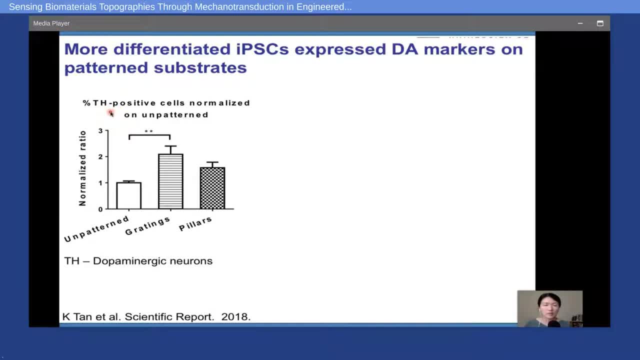 information. we examine the expression of tyrosine hydrogenase, which is a marker of the primomunergic neurons, On grating. we observe that there is a significantly higher percentage of tyrosine hydrogenase positive cells on gratings. We also have higher TH-positive. 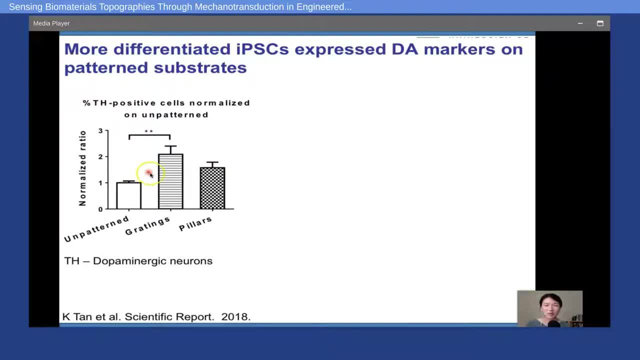 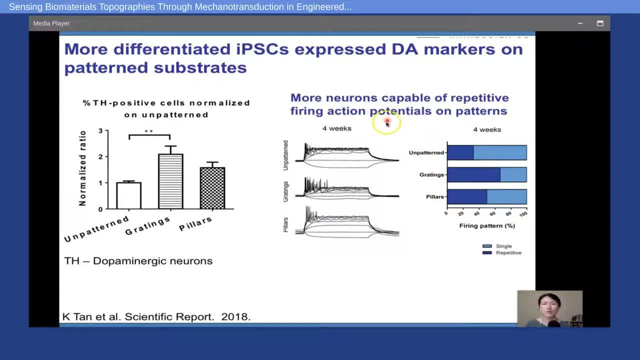 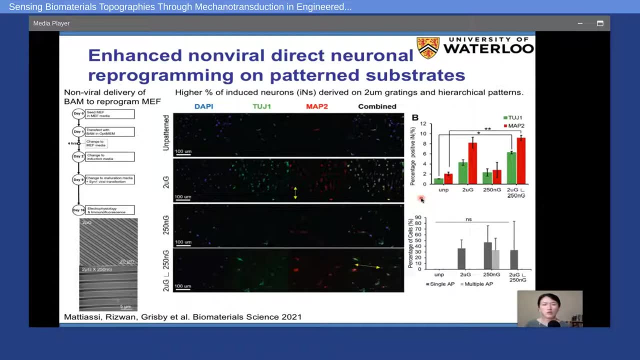 or the electrophysiological functions of the neurons. we find that there are more neurons capable for firing repetitive action potentials on the patterns, on both the gratings as well as the pilars pattern. In our recent work we have shown that using 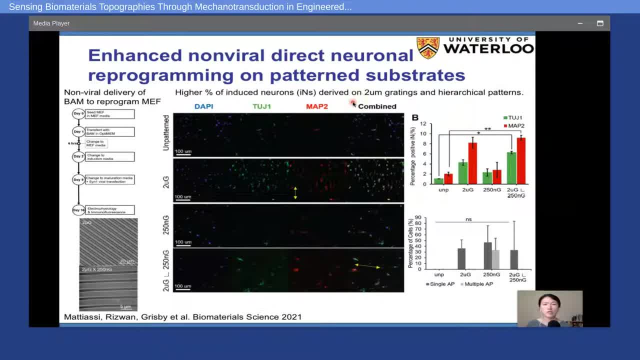 a topography pattern. it can also enhance the derivation of induced neurons by using non-viral, non-viral gene deliveries to reprogram mouse embryonic fibroblasts into neurons. In this study we reprogram mouse embryonic fibroblasts. 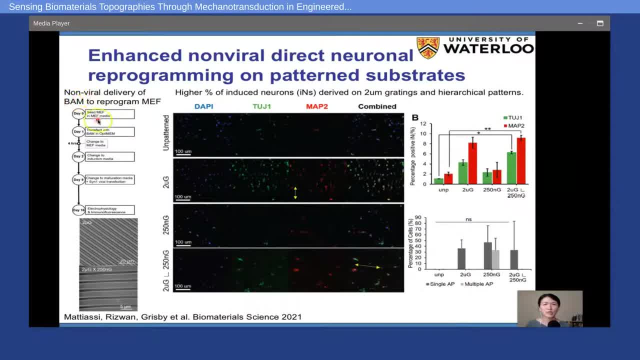 by delivering the BAM factor to the cells with a non-viral gene delivery, with a polyplex delivery, with only one dose of polyplex delivery. So after around two weeks we observed a higher percentage of cells' expression, of cells' expression. 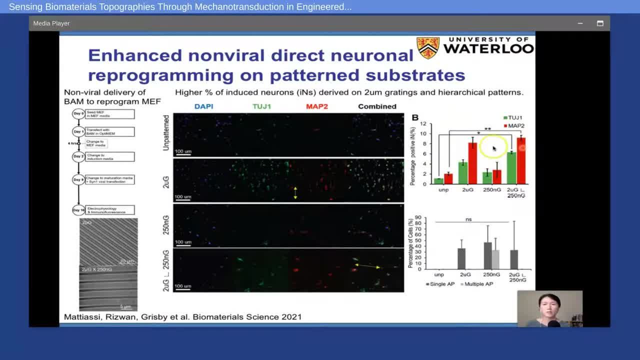 of cells' expression, both TUJ1 as well as MAP2, with the highest expression on a hierarchical pattern, which means that we have 250 nanometers gratings, patterns in parallel on top of a 2 microns gratings On the 2 microns grating. 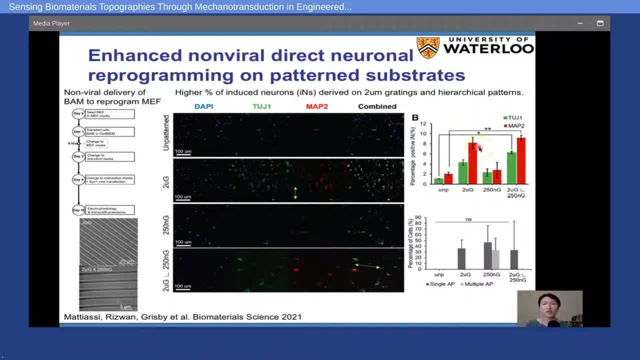 and the 250 nanometers gratings. we also have an increased TUJ1 expression and MAP2 expression. So again, TUJ1 is a marker for a panneuronal marker and MAP2, the myosin-associated protein 2,. 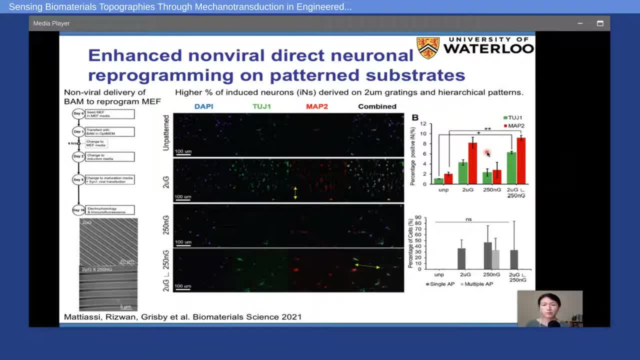 is a marker for neuronal maturation. We also measure the electrophysiology activity or functions of the neurons And we find that we could detect cells with single action potential and multiple action potentials when the cells are derived on a gratings pattern. But we couldn't detect 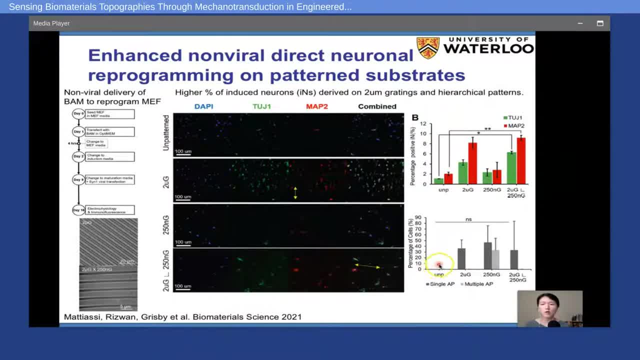 any electrophysiological activity in the cells on a patterned substrate. So this also gives us supporting evidence that topography substrate, especially grating substrate, could enhance the derivation of neurons or neuronal differentiation. However, what is the mechanism behind it? 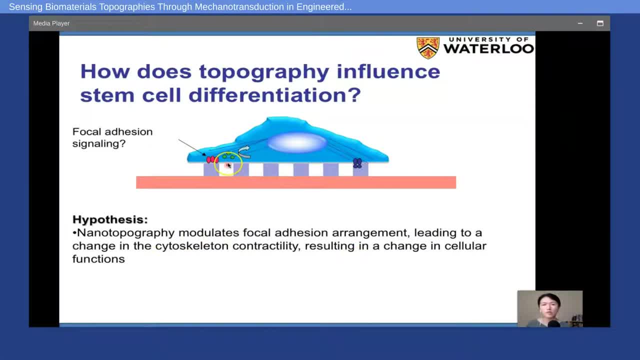 So we hypothesized that nanotropography could modulate focal adhesion arrangement, which will lead to a rearrangement or change in the cytoskeleton contractility And it could, as a result, change the cellular function. We start looking into the problem. 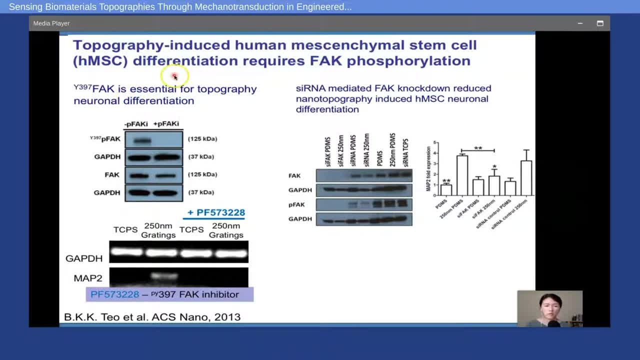 by using human mesenchymal stem cell, specifically the neuronal differentiation of human mesenchymal stem cell, as a model cell system to investigate what is the mechanism behind topography-induced differentiation, As during the differentiation we observed a high expression of phosphorylated focal adhesion. 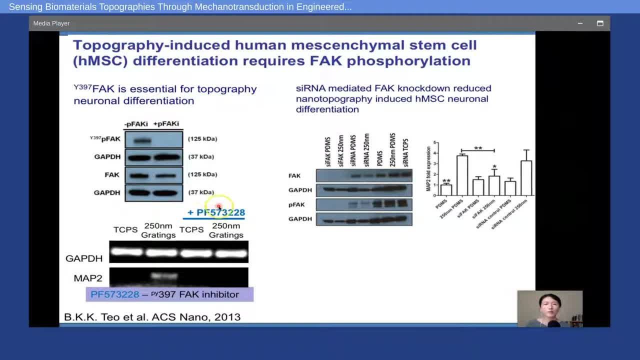 kinase. we would like to apply a small molecule inhibitor, the PF573228,, to specifically inhibit the phosphorylation of the tyrosine-397 site of focal adhesion kinase. Using this small molecule inhibitor, we can inhibit the phosphorylation of the tyrosine-397 site of FAK. 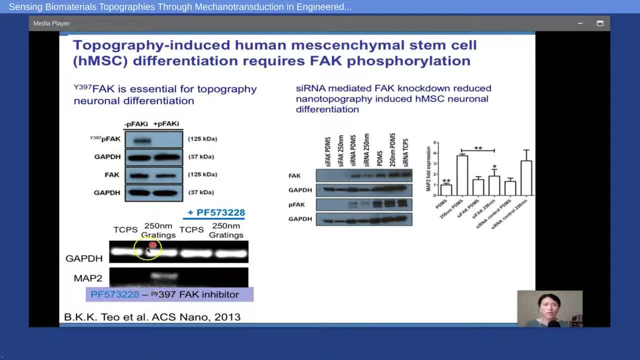 And we find that the neuronal marker that usually is upregulated by the topography-induced differentiation is abolished when we inhibit the phosphorylation at the tyrosine-397 site. To further show the rules of focal adhesion kinase played in the topography-induced 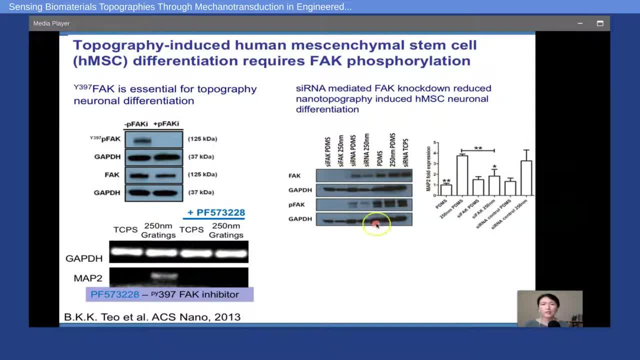 differentiation. we also use SRNA to lock down the FAK expression in the human mesenchymals themselves. Indeed, we find that with the knockdown of the focal adhesion kinase we also observe a significant reduction in the neuronal marker expressions that we usually will. 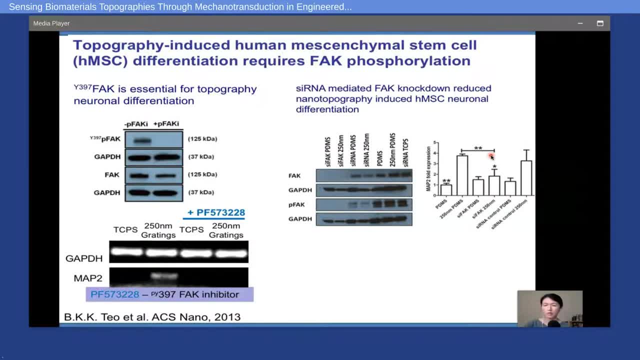 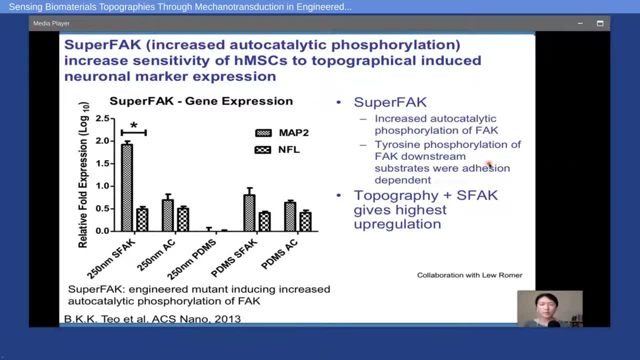 see in the topography-induced differentiation. In a collaboration with our collaborator, Professor Lou Romer in Johns Hopkins University, we use SuperFAK, which is an engineered mutant inducing an increased autocatalytic phosphorylation of FAK. Using SuperFAK, we find that it 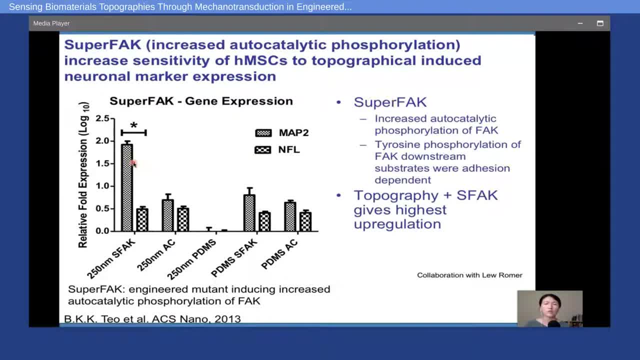 actually increased the sensitivity of the human mesenchymal stem cells to topography sensing, In which the topography-induced neuronal marker expression is significantly higher when it's exposed to the topography. So it further shows the significant involvement of focal adhesion kinase. 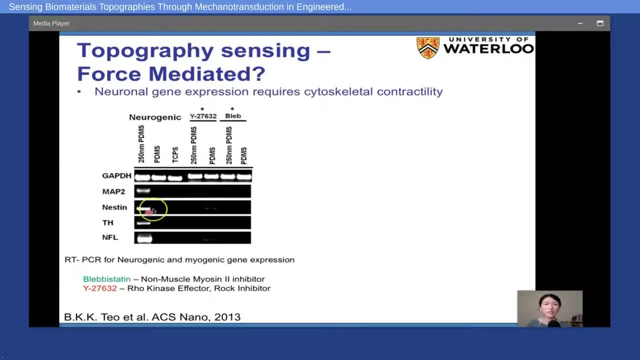 in the topography sensing. Another question that we would like to ask is: what is the rule of the force sensing in terms of the force-mediated signal by the cytoskeleton contractility? So in this experiment we also applied two other small molecule inhibitor. 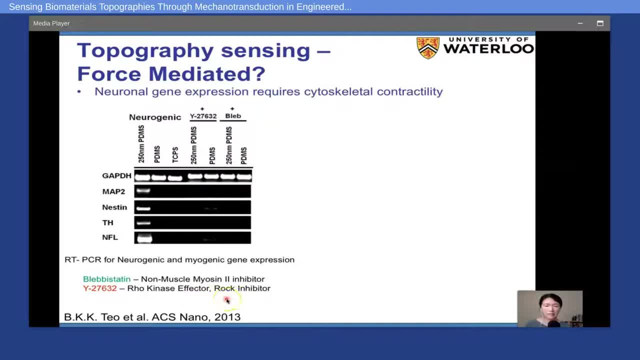 The Y compound, which is the lock inhibitor inhibiting the role kinase effector, as well as buprenorphine, which is an inhibitor for non-muscle myosins too, When we apply these two inhibitors to inhibit the cytoskeleton contractility. 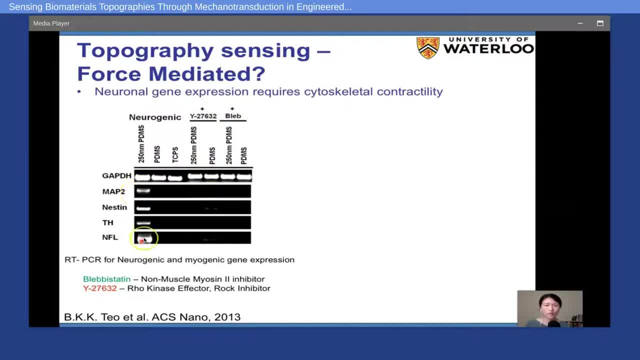 we see the neuronal marker that usually expressed in the cells undergoing topography-induced differentiation. those neuronal markers' expression is being abolished. It shows that the topography-induced differentiation does require cytoskeleton contractility. We would also like to investigate the involvement of cytoskeleton contractility. 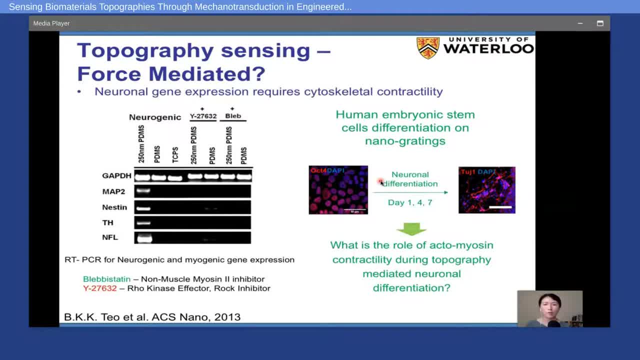 in the embryonic stem cell differentiation, or nanotopography. My other student, Zolila, has taken this work and she investigates the role of ethyl myosin contractility during the early phase of topography in mediated neuronal differentiation. 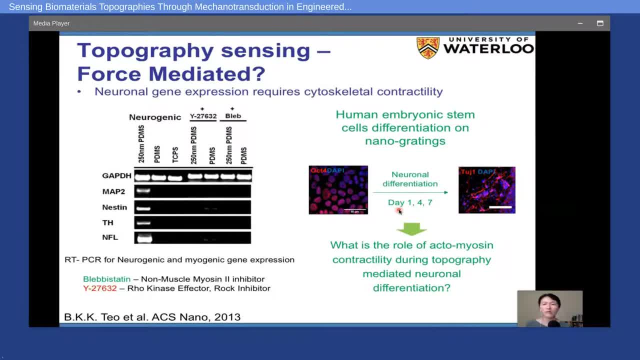 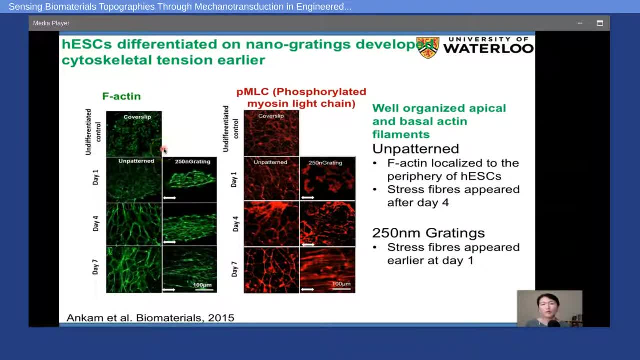 and she looked at the expression in day one, day four and day seven after the neuronal differentiation has started. So in polyprosense stem cells, in embryonic stem cells, when they are undifferentiated they have very low expression of stress force. 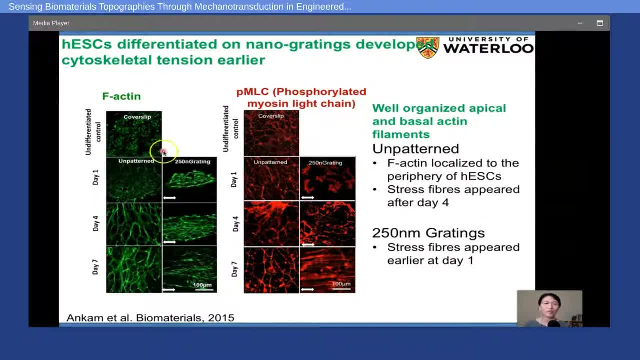 stress fiber or cytoskeleton contractility. So both advectrin expression as well as the phosphorylated myosin light chains expression is quite low During the differentiation process. the formation of stress fiber as well as the phosphorylated myosin light. 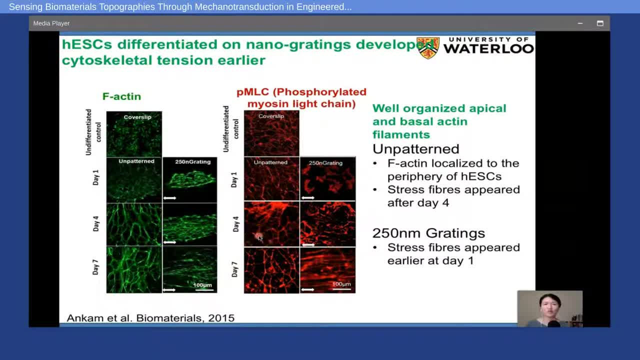 chains, expression will increase as the cell starts to differentiate. So during this process we find that the cell's culture on the 250-meter nanogratis, on the 500-meter nanogratis, will have stress fiber appeared as early as day one. 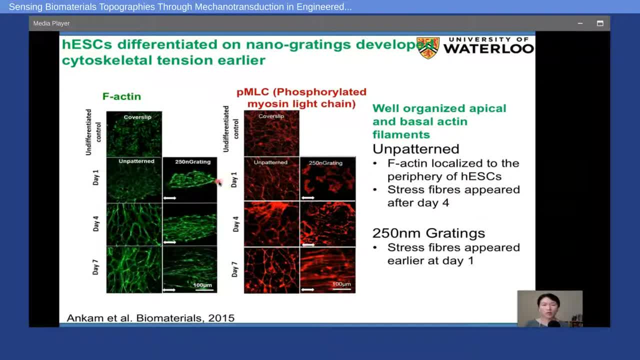 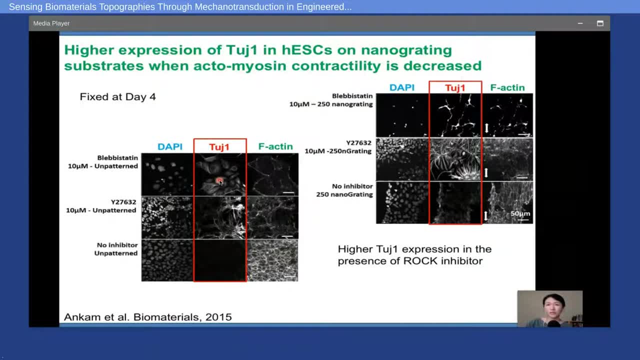 So the cytoskeleton contractility developed much earlier on the nanogratins. Very interestingly, when we applied the inhibitor, the Y compounds, to the rock inhibitor, we actually observed with the presence of rock inhibitor we have a higher expression of TG1. 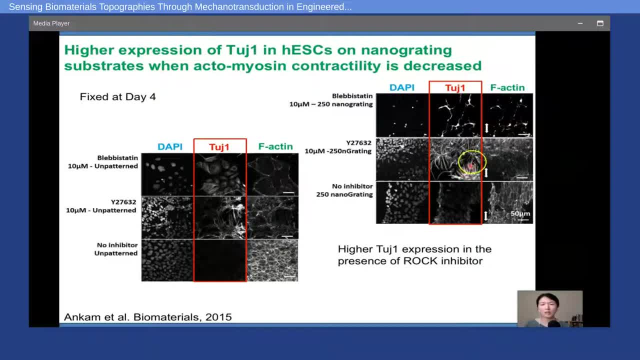 in the human embryonic stem cells, quite showing on the nanogratins. And in this case it means that when the ectomyosin contractility is decreased, we actually have a higher expression of the neuronal marker. Meanwhile, in the presence 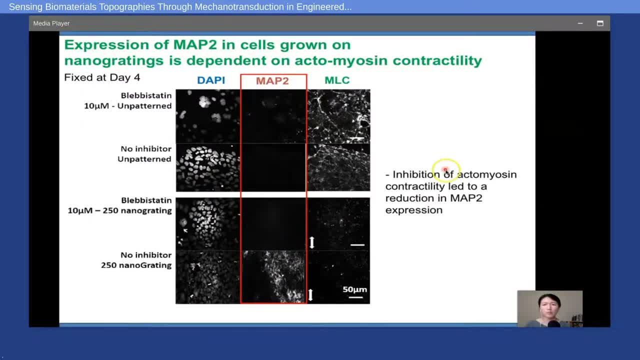 of pipistentin. when we inhibitor, we have a higher expression of TG1 in the cell and it actually leads to a reduction in MAP2 expression. So these two data seems to be contradicting, But if we think about it, this is actually agreeing. 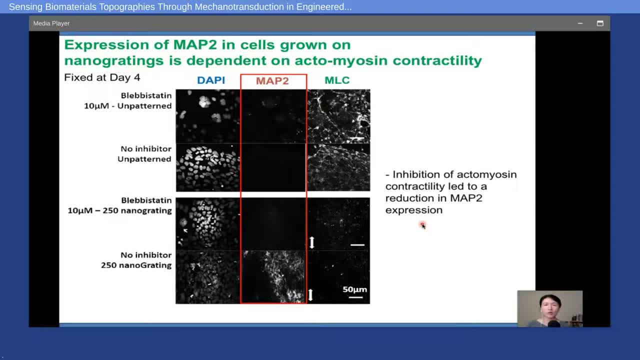 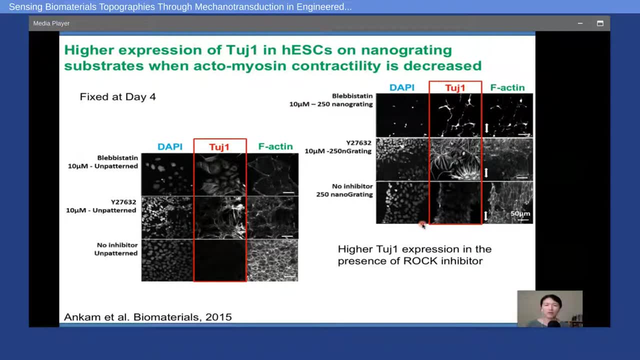 with what other researchers has find in the literature as well. In the literature other researchers has find that using a soft substrate will help to enhance and induce neuronal differentiation And in a soft substrate the cells will have a more, will have developed a lower. 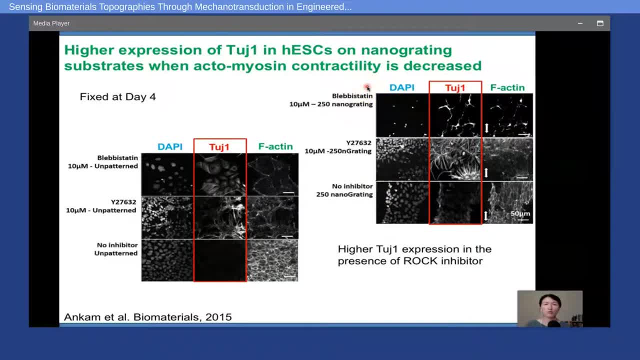 ectomyosins contractility in response to the softer environment, which is similar to when we apply a low dose of Y compounds to lower the ectomyosins contractility And, in response, the combination of that walk inhibitor with the nanogratings. 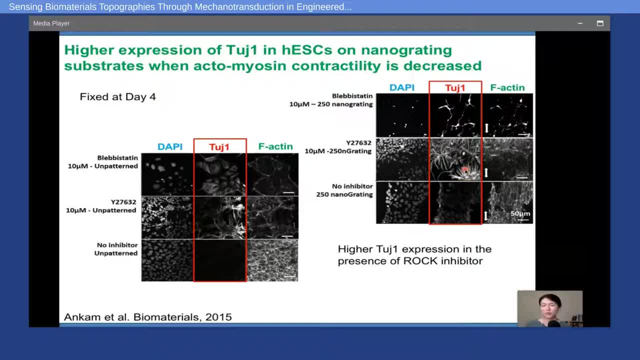 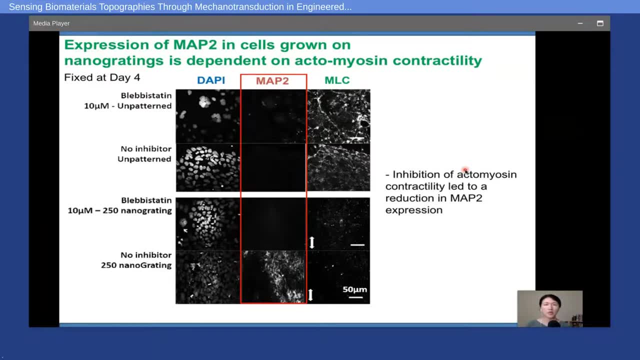 we observe a higher expression of TuJ1.. However, as what we have observed in our human mesenchymal stem cell study, as the ectomyosins, contractility is needed for the topography mediated differentiation. if we inhibit the ectomyosins. 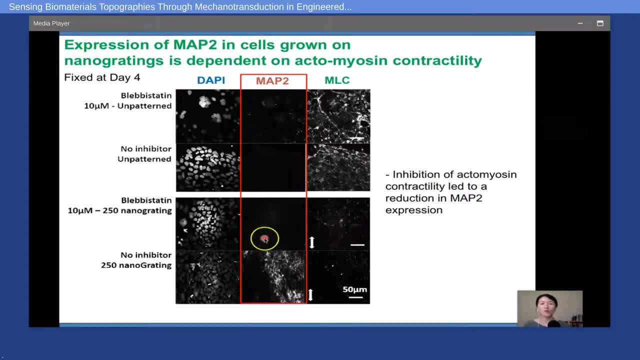 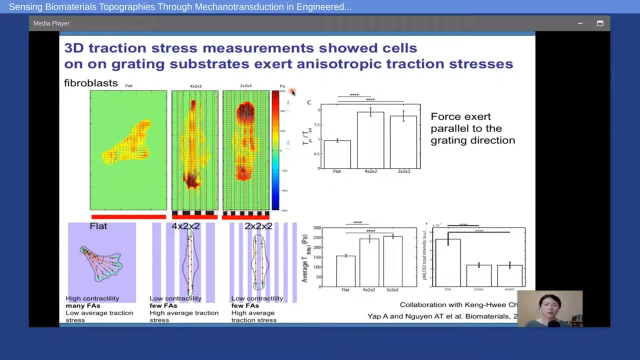 contractility. by pipistatin, we will not be able to observe the maturation of the neurons and the expression of MEP2.. So when we are talking about the expression of MEP2, we are talking about the cytoskeleton contractility we would like. 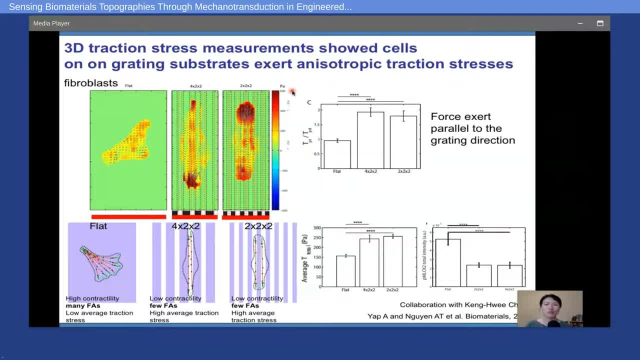 to quantitatively examine the ectomyosins, contractility and the traction force of the cells culture on the gratings. In collaboration with our collaborator, Dr King Wei-Chim in Bao Informatics Institute in Singapore, we have developed this 3D. 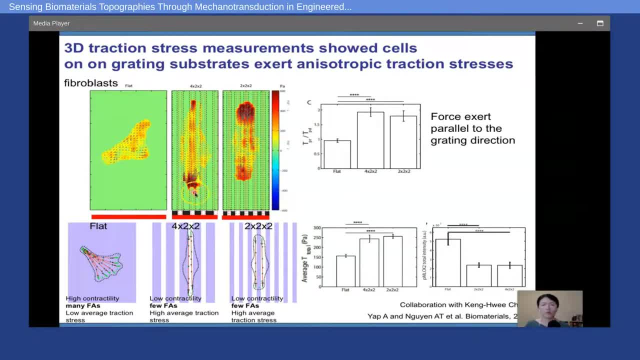 traction stress measurement system on two microns gratings. So first we observed that the cells on these microgratings exert a significantly higher force, that is, in the parallel directions to the gratings And other interesting study observation that we have is that the cells actually 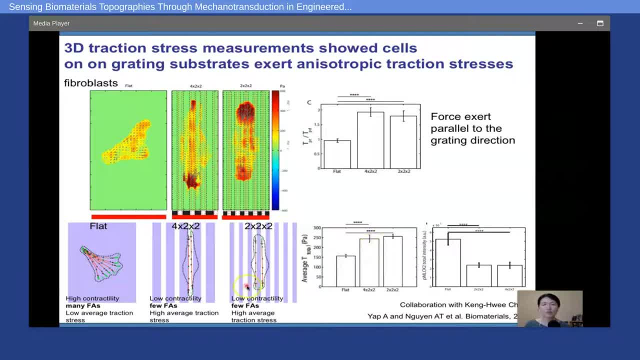 exert a higher traction force on each of the focal adhesion. So, two slides ago, we mentioned that the lower contractility will help to enhance neuronal differentiation. Indeed, this is also what we observed, or what we speculate, Because when the cells are 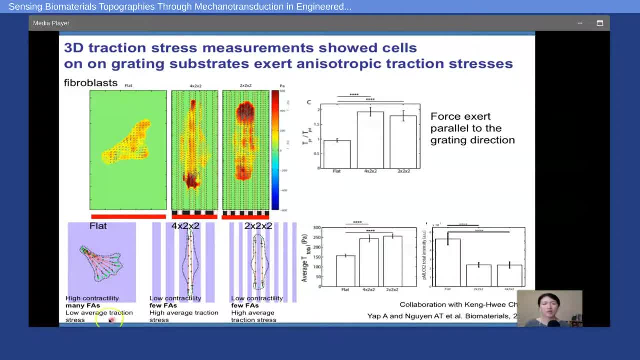 cultured on a flat or impactant substrate we see many more focal adhesion, But on the grating substrate we observe fewer number of focal adhesion. So although the traction force per each focal adhesion is increased, when we investigate the overall contractility. 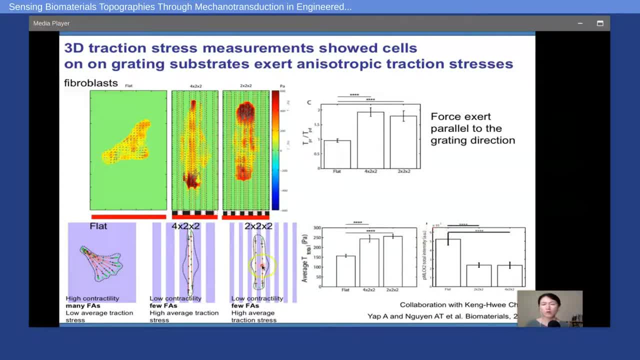 we actually find the overall contractility is lower in the cells on the gratings, which also agree with our speculations that the grating substrate will lead the cells to have a lower contractility, which also is one of the reasons why it could contribute. 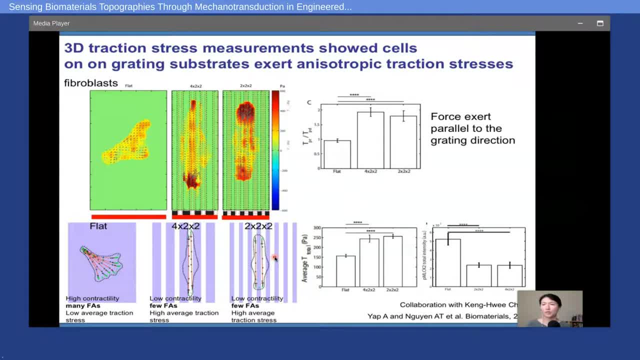 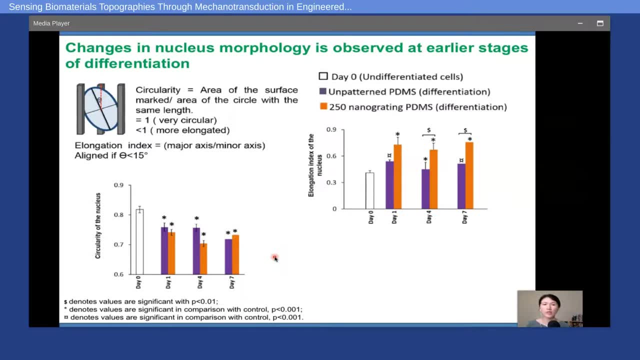 to the enhancement in the gratings. We also hypothesized that the change in the cytoskeleton may also affect the gene regulation in the nucleus. So we also looked into the nucleus morphology at the early stage of differentiation. So on the cells cultured, on the nano and macros gratings. 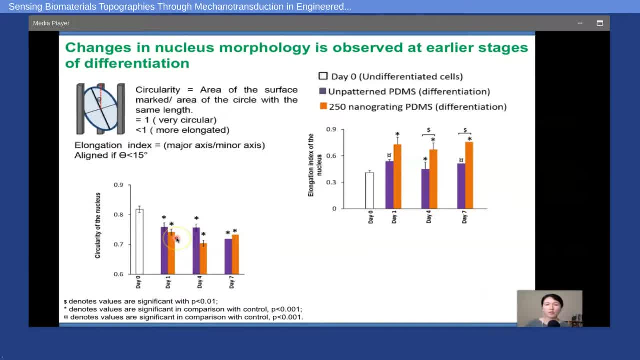 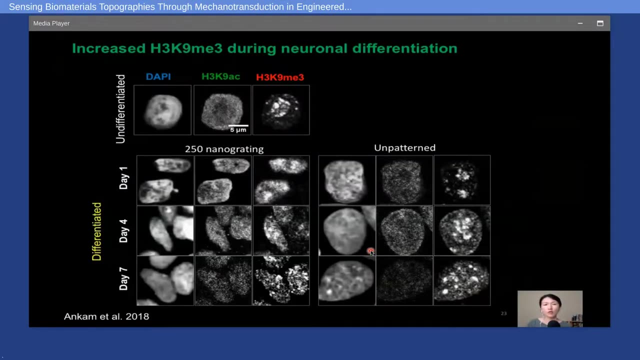 we find that the nucleus also significantly elongated on the gratings substrate And the nucleus is also aligned along the gratings direction. We also observed that there's an increased X3K9Me3 expression in the early phase of the neuronal differentiation. 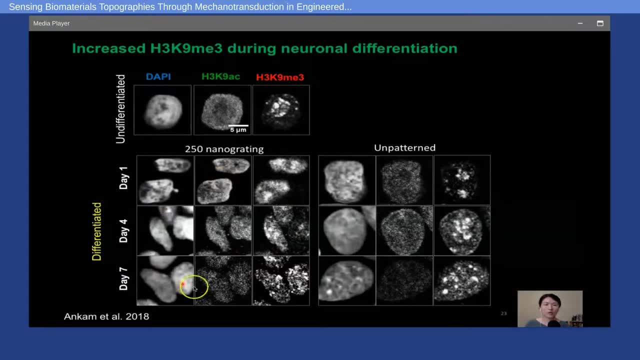 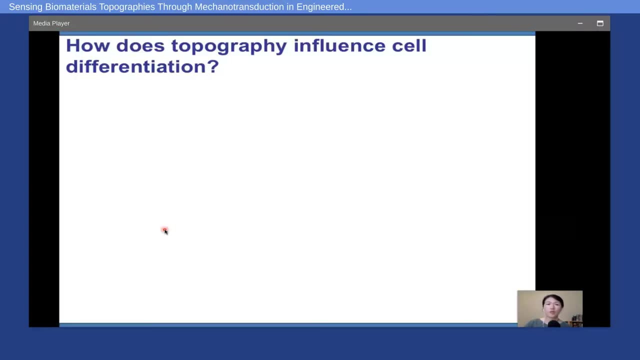 when we culture the embryonic stem cells on 250-meter nanoskeleton. So, in summary, we speculate how topography influence cells, differentiation or cell behavior. The true mechanism as followed: Topography signals are transduced through vocal adhesion, kinase signaling. 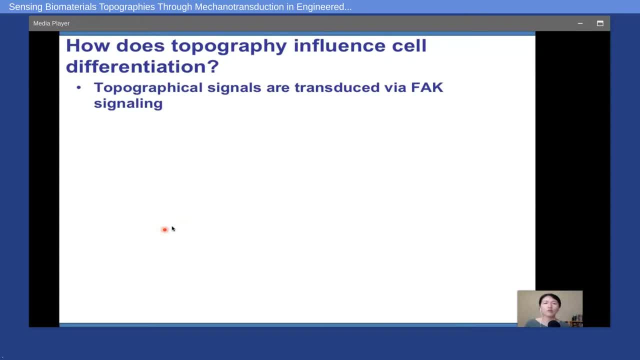 And topography induced differentiation is mediated by ectomyelins contractility, And the topography induced differentiation is mediated by ectomyelins contractility. And we also found that the topography induced differentiation is mediated by ectomyelins contractility. 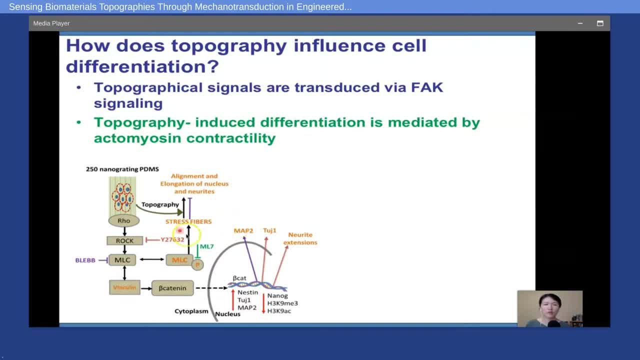 And both this ectomyelins contractility as well as the vocal adhesion signaling is important in topography sensing. When we decrease ectomyelins contractility of the cells it could enhance the neuronal lineage commitment. So there's more TUJ1 positive. 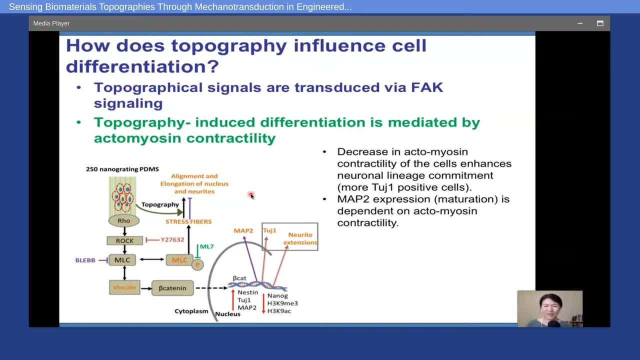 cells. However, if we inhibit the ectomyelins contractility, it could also inhibit the neuronal maturation. So MAP2 expressions- the maturation of the neurons is actually depends on ectomyelins contractility. With using a 3D traction force,